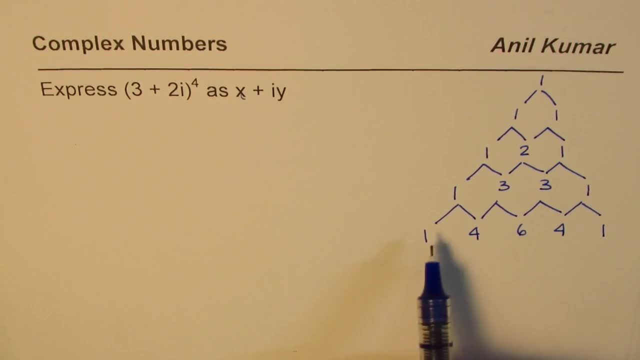 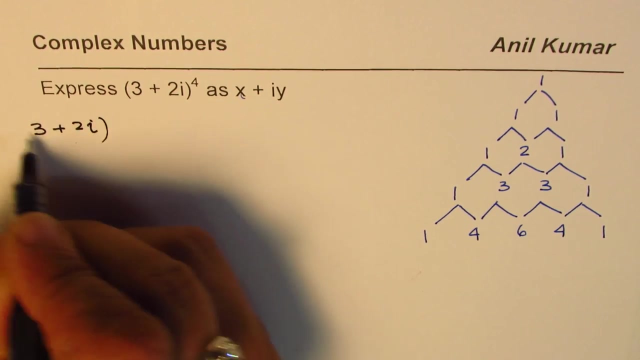 1. see this expression. now, this is a fourth row for us, which represents the coefficients for expanding a binomial term. right, so we'll have five terms. we could write 3 plus 2i to the power of 4 as equal to so here the first term is 3. 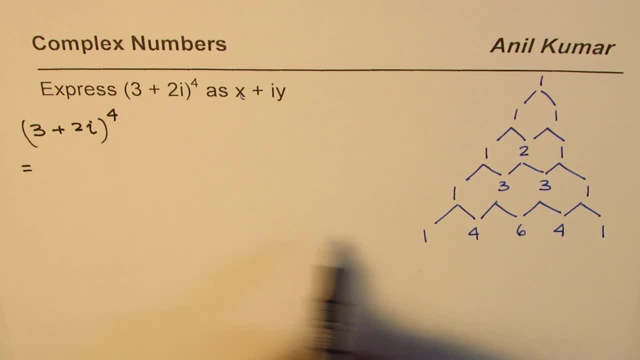 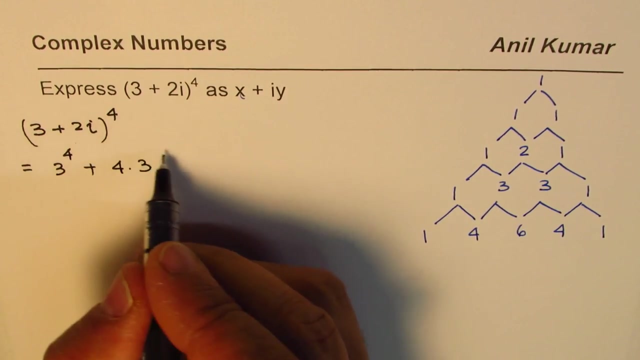 the second is 2i. the coefficient will be 1. powers will be: sum of powers will be 4, so I could write this as 3 to the power of 4, plus. next time the coefficient has to be 4, right? so we like four times 3 to the power of 1, less than. 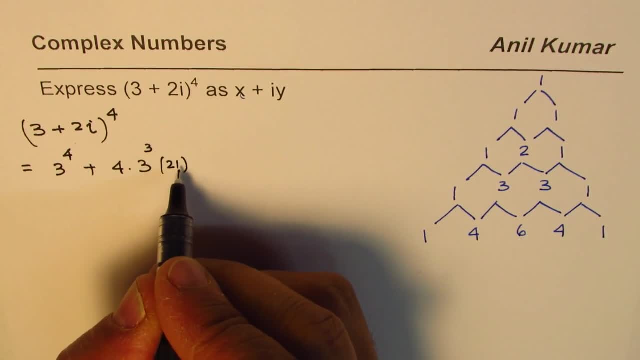 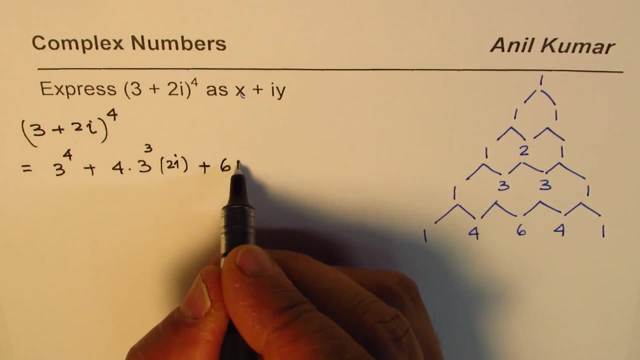 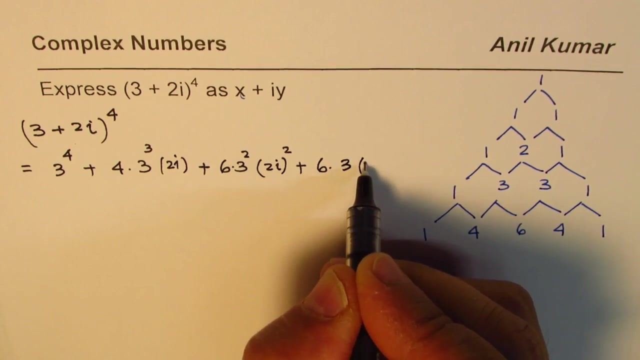 4 and the second term, which is 2i for us will have power of 1. now plus 6 will give us 3 square, and square of 2i plus this power will reduce by one right. let me write dot here. so we have plus six times three times two. i cube right. 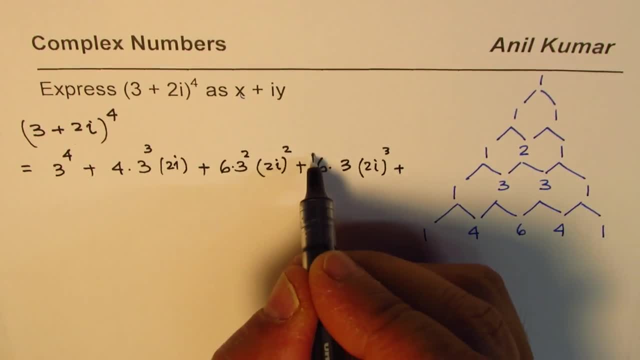 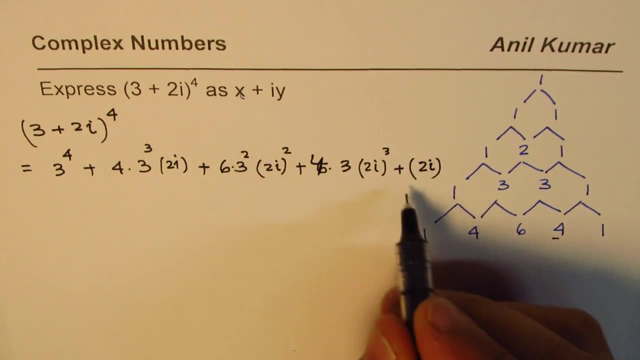 and the last term will. i'm sorry, this should be four, sorry, this coefficient four. the last term will be two. i to the power of four. coefficient is one. i'm not writing that, not required. so what we get here is three to the power of four. you can use the calculator at this stage. three to the. 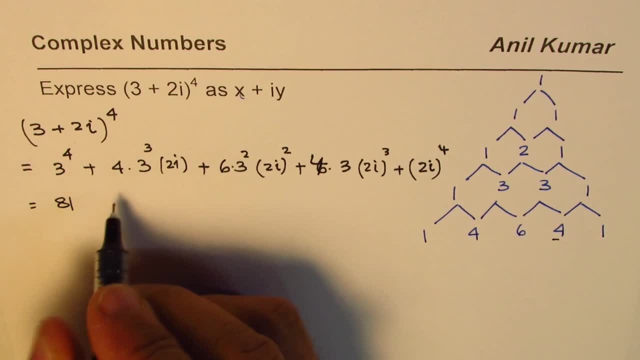 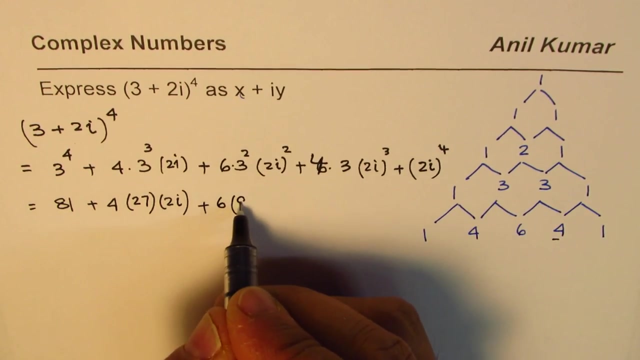 power of four is nine times nine, eighty one. let me write eighty one here now. here we get four times three, cube. let us do it in two steps. which is 27 times two, i okay. plus six times three, square is nine. square of this is four: i square is okay. now. the next term here is plus four times three. 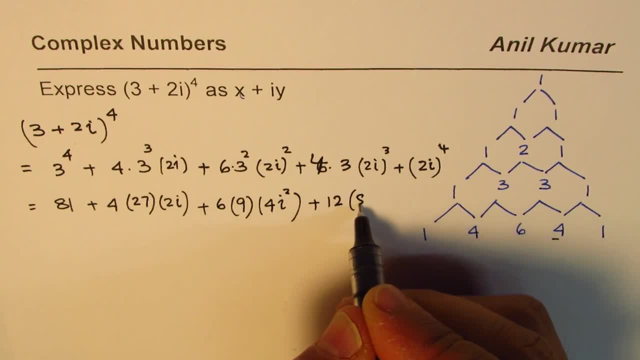 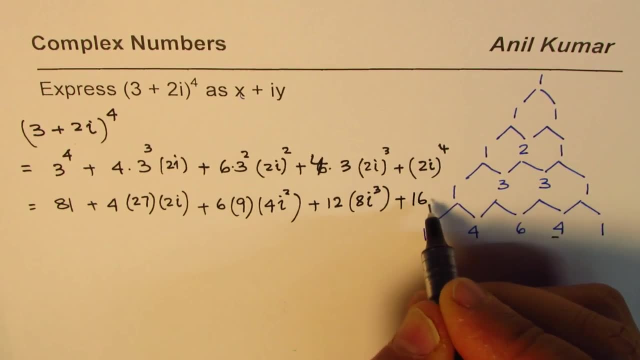 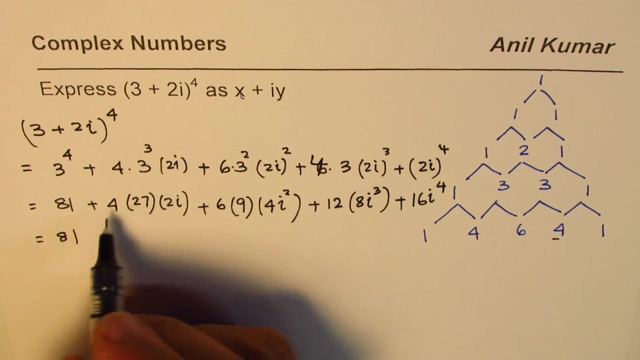 is 12.. two cube is eight, i cube right. plus two to the power of four, that means 16 i to the power of four, correct, okay, so that gives us 81. now we can multiply these numbers: four times two is eight. eight times seven is 56. five eight times two is eight and five is 13. i, i square is minus one. so 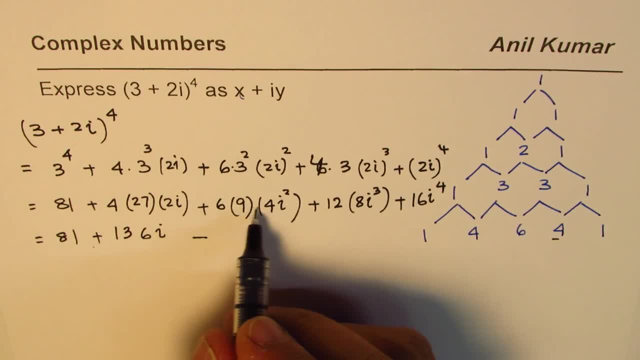 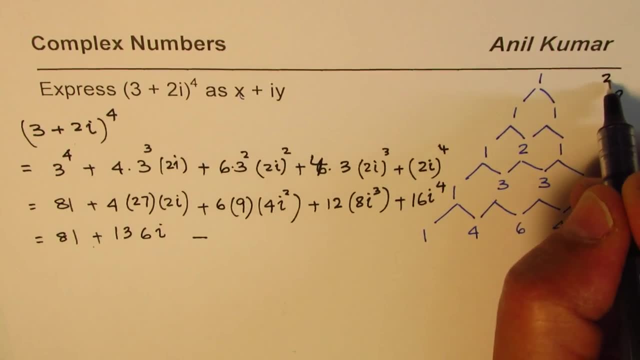 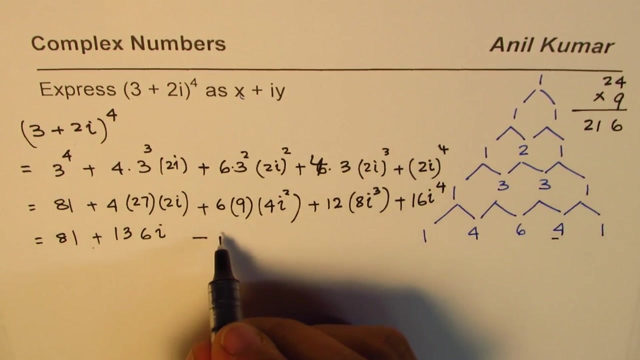 and then we can have six times nine, right. so let's do six times nine. so nine. six times four is 24. let's multiply that by nine, nine times four. thirty six, three, nine times two, eighteen. so two, one, six. okay, two, one, six, i square minus one. now, in this case 12 times eight, so you get plus. well, i cube is minus i. 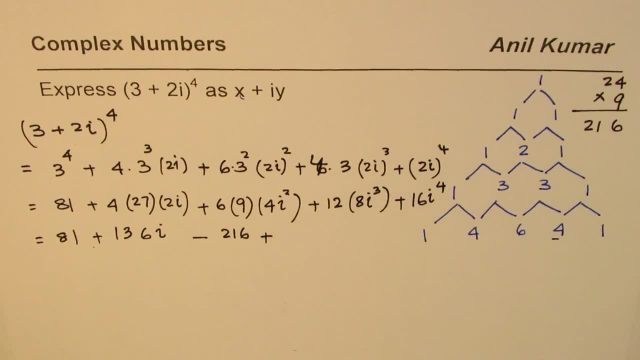 should write minus here. we'll put minus i here, as you know. uh, let me rewrite here: i square is minus one, i cube is minus one times i, which is minus i, and i to the power of four is one. so we are going to use this also while expanding, is it okay? now? 12 times eight, eight times two is sixteen, six one. 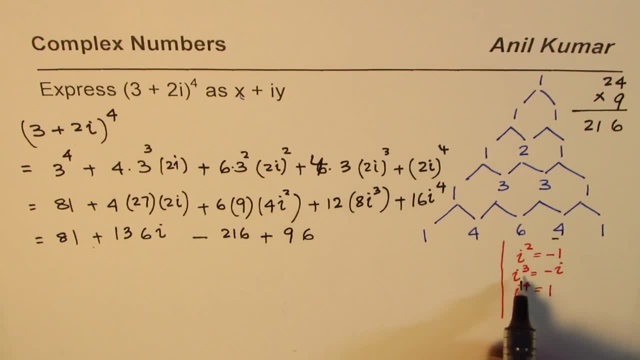 ninety six. right, i cube, so i cube is minus i, so i'll write minus i this time. i, to the power of four, is one, so we get plus 16. you see that. so we have two terms, with i and others are constant real numbers. we'll add them up so we have 81. this is plus 136, i minus 216. 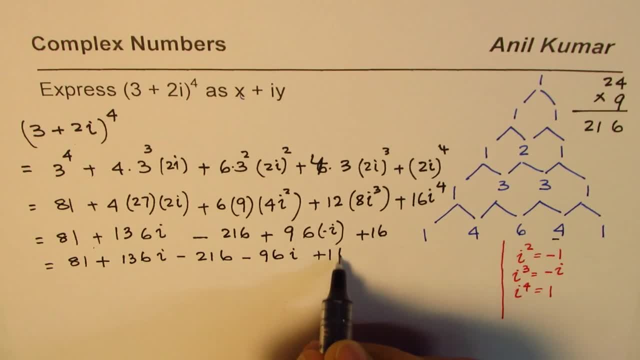 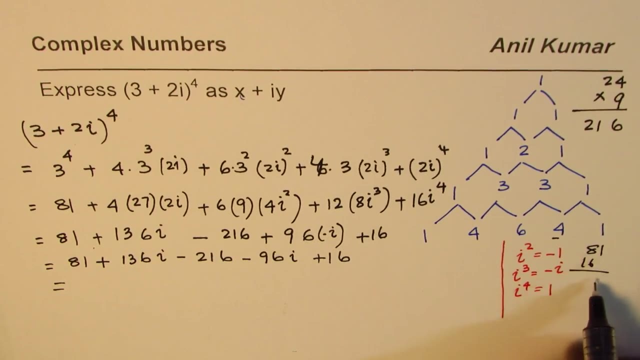 here we have minus 96, i plus 16, right? so we can combine the numbers and: and so we have 81 plus 16, which is 797. we'll take away 97 from 216. we have 216, take away 97, so that gives us 9, 10 gives us 1, 1, 1, 9, so we get here minus. this is negative number, right? so we did. 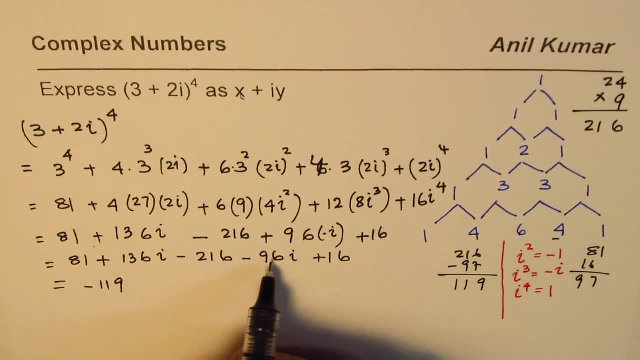 kind of reverse minus 1, 1, 9. as far as the i terms are concerned, we'll take away 96 from 136, 6 take away, so we have plus. this plus is bigger: 13 take away 9 is 4, so we have 40, 40. i. 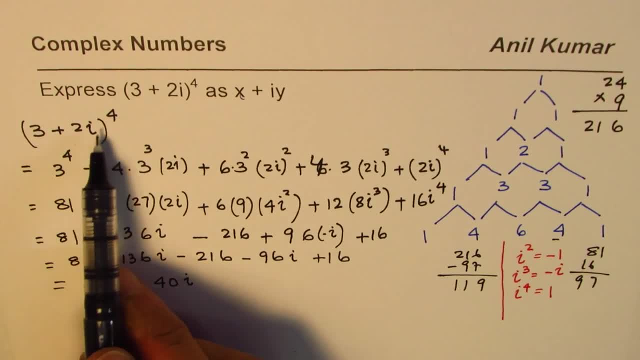 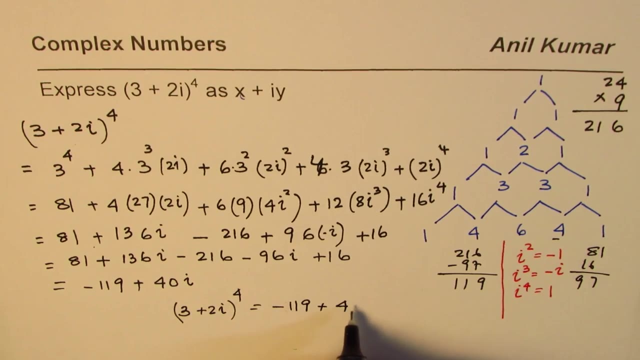 so the expression 3 plus 2 i to the power of 4 can be written as minus 1, 1, 9 plus 40 i. so let me rewrite the answer, which is: 3 plus 2 i to the power of 4 is equals to minus 1, 1, 9 plus 40 i.